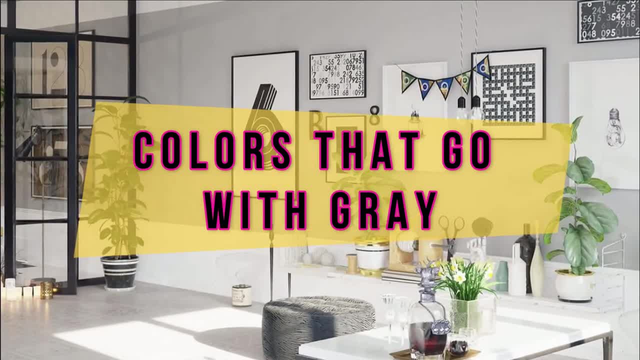 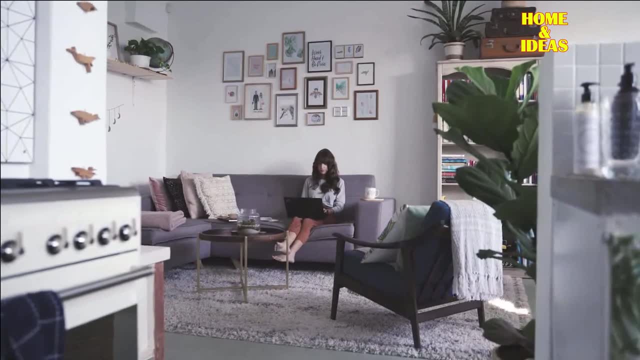 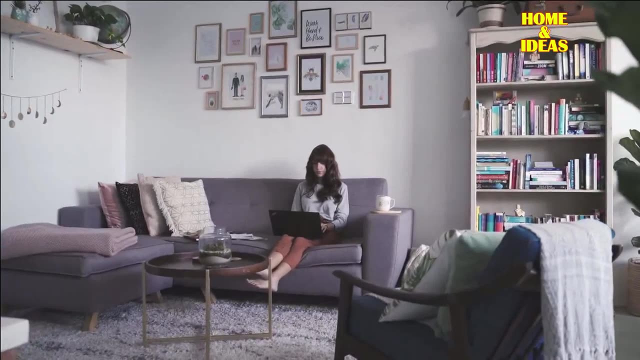 What are the colors to combine with gray? This is a question that very often afflicts us, especially for those who are struggling with the furnishing and decoration of their home. Gray is anything but a characterless shade If you, too, have decided to set this nuance in your home. 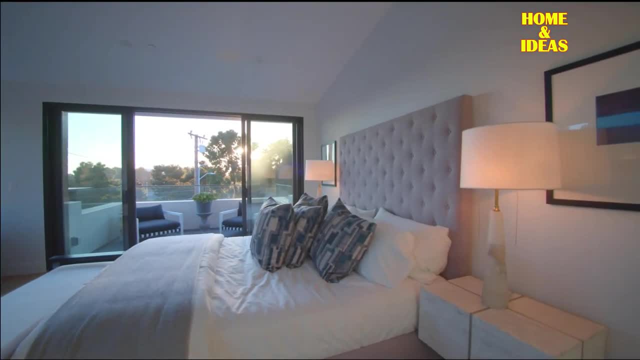 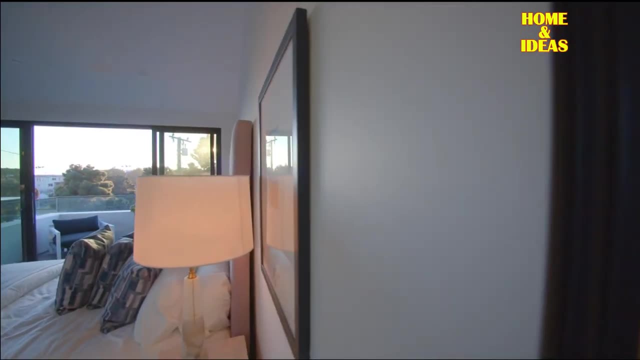 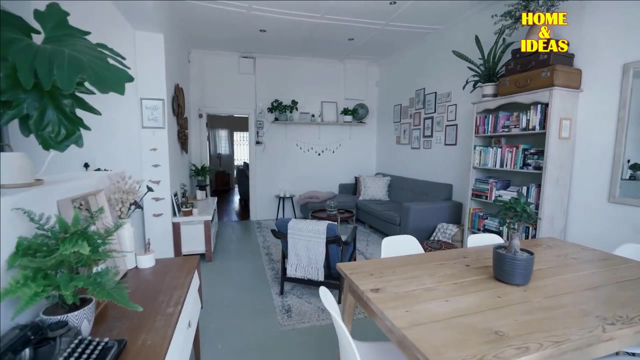 you will undoubtedly have made the right choice. In this way, it is possible to give elegance and sobriety to the space. What does the gray color symbolize? Gray is a cross between black and white. Very often it is underestimated, but this color has. 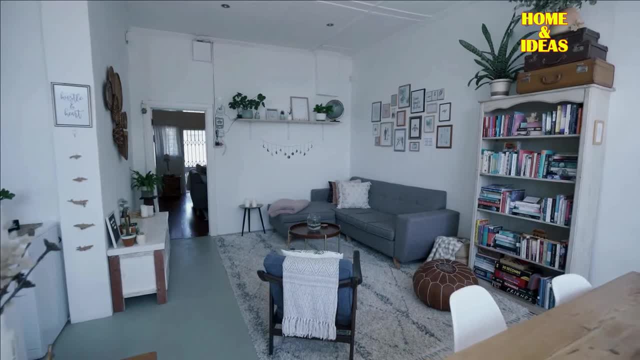 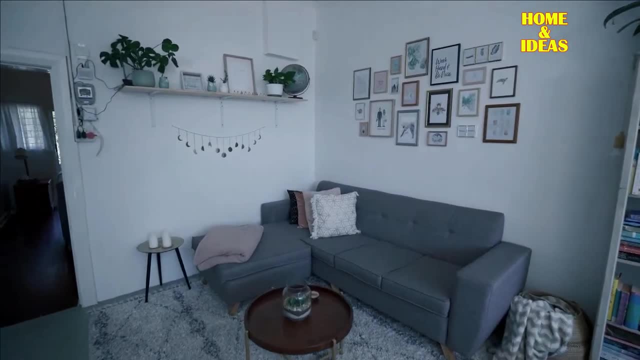 many properties that can completely change the look of your home. Its symbolic meaning is very profound. Ah can mention it as safety and stability. All the more reason to adopt it also in the decoration of the house. It is a symbol of intelligence and maturity. 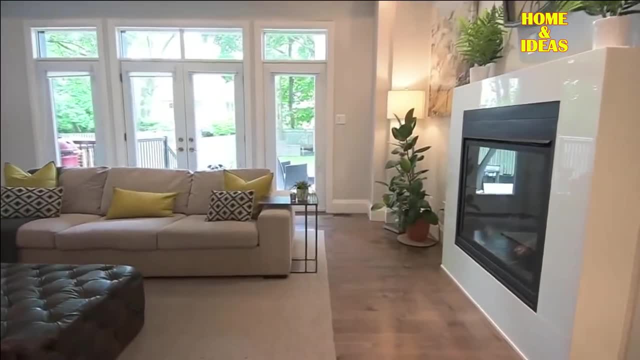 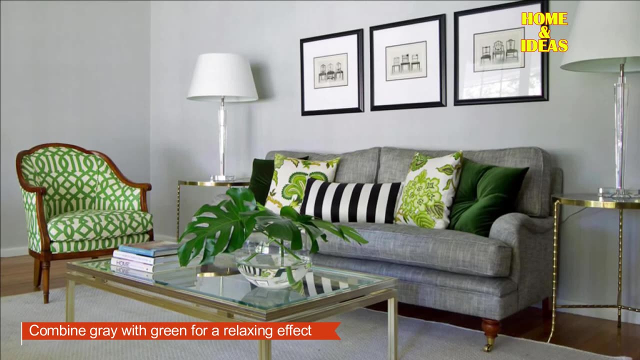 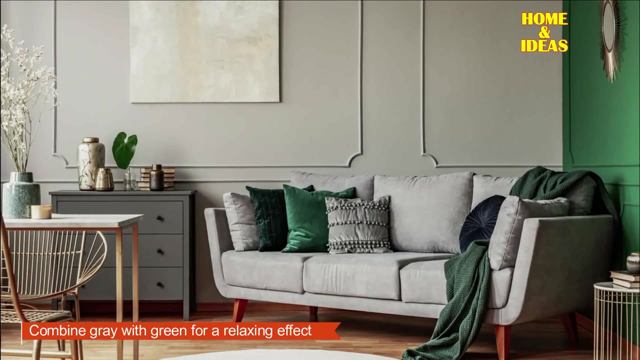 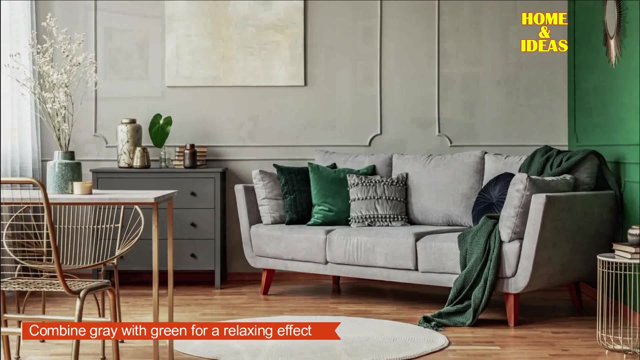 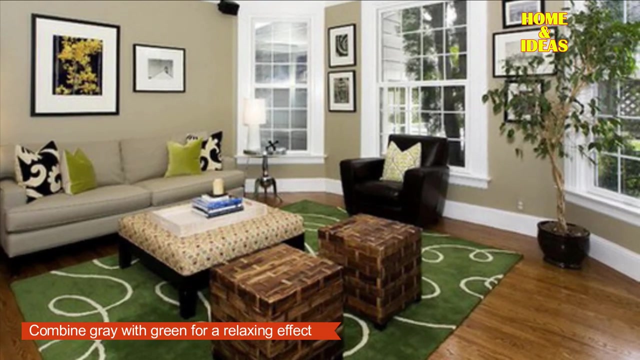 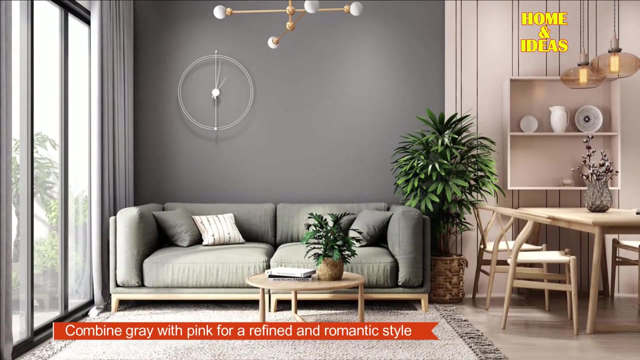 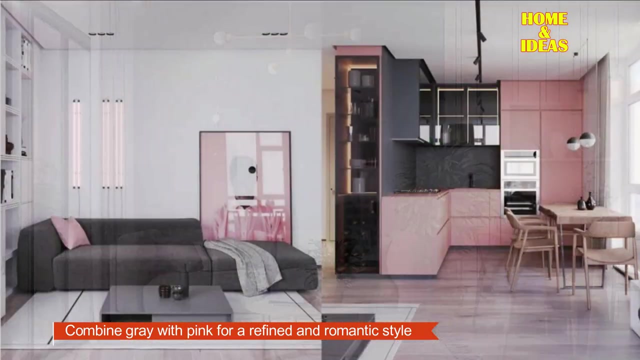 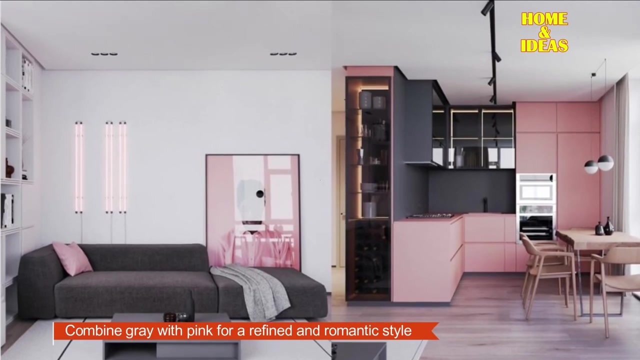 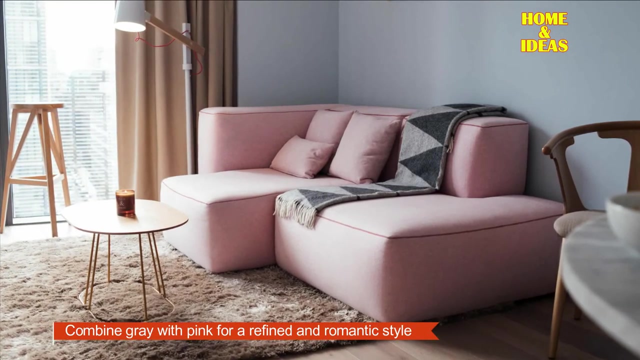 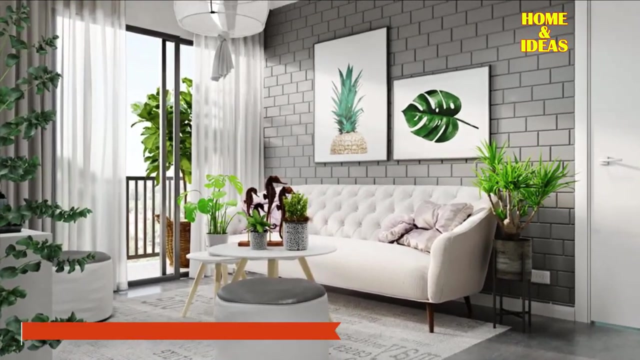 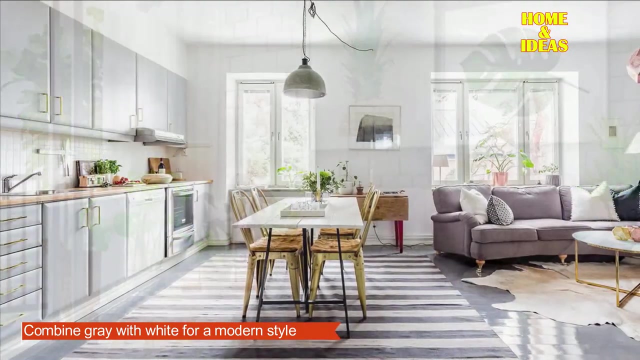 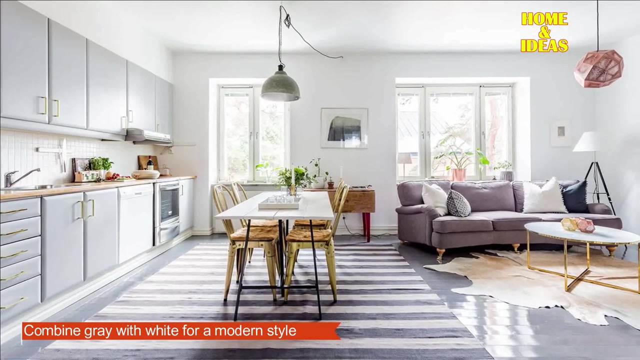 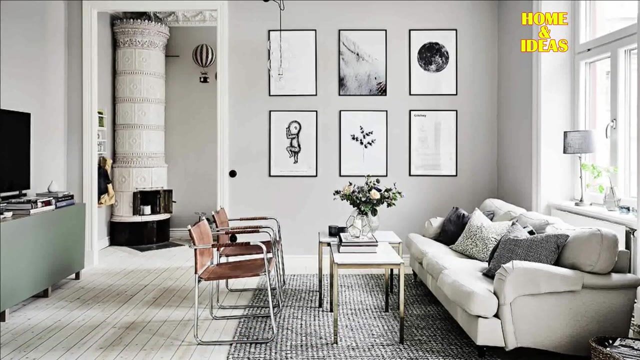 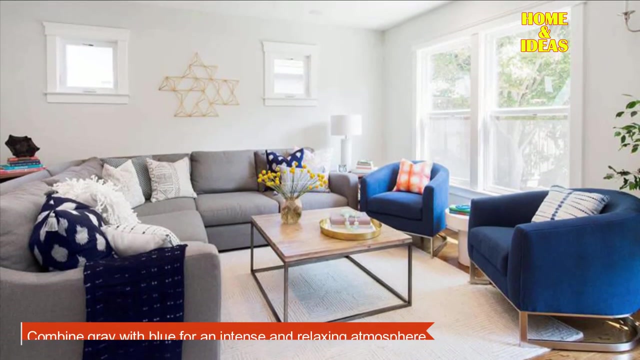 Here are some colors that go with gray for your interior design. Combine gray with green for a relaxing effect. Combine gray with pink for a refined and romantic style. Combine gray with white for a modern style. Combine gray with blue for an intense and relaxing atmosphere.